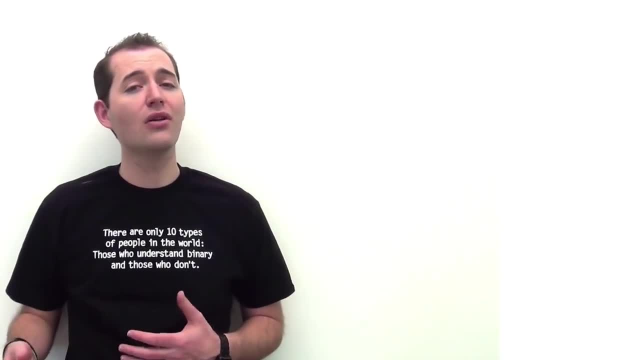 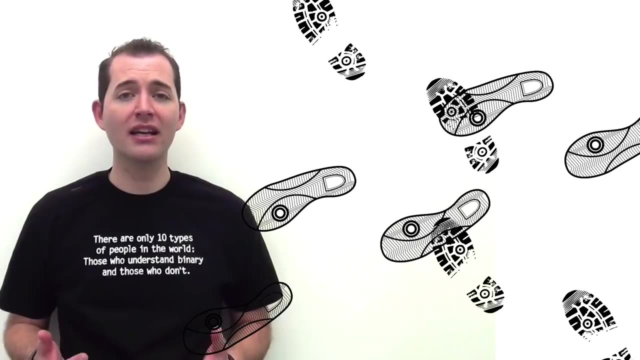 Let's compare the law of crosscutting to tracks in snow or in sand. In this scenario, the older tracks will be covered by younger tracks. This allows us to determine the relative age of those tracks, where those that are on top or are not covered by anything are. 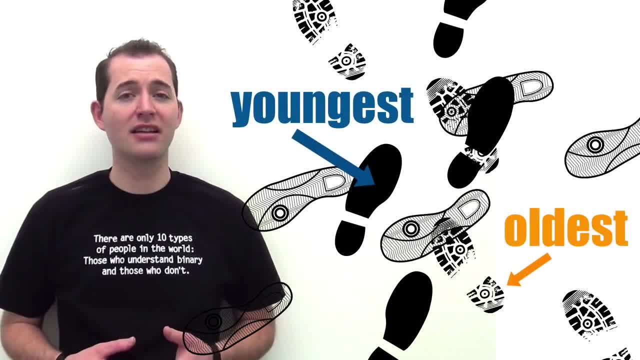 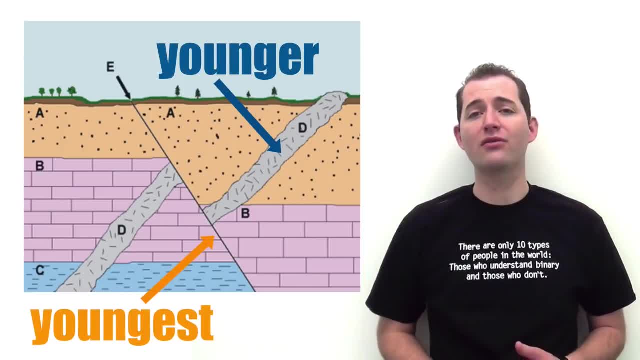 the youngest, and those that are covered by the most are the oldest. This is also true with any rock sequence with crosscutting features. Those features are younger than all of the rocks they cut. Finally, let's look at the law of inclusions, or, as it's also known, the law of included. 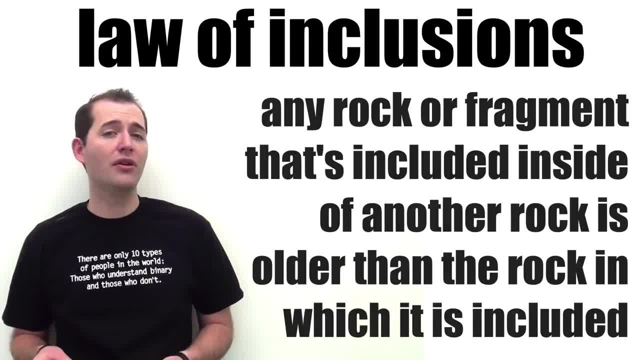 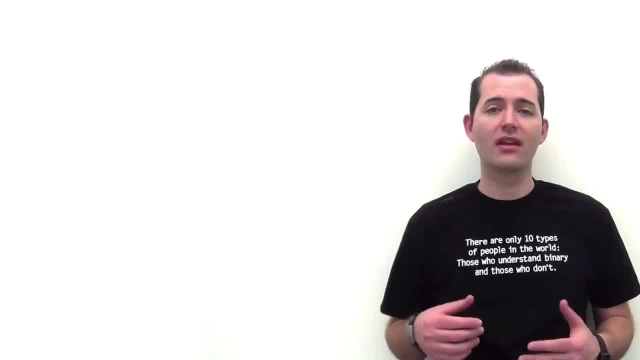 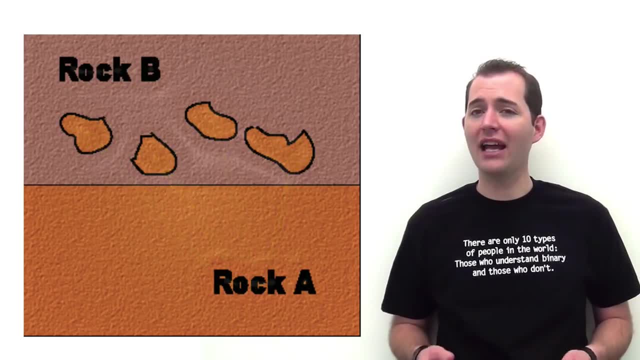 fragments. This law states that any rock or fragment that's included inside of another rock is older than the rock in which it's included. For example, if we look at this diagram, pieces of rock A are inside of rock B. This means that rock A is older and rock. 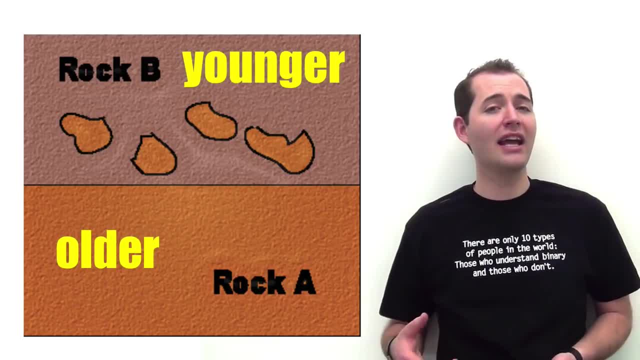 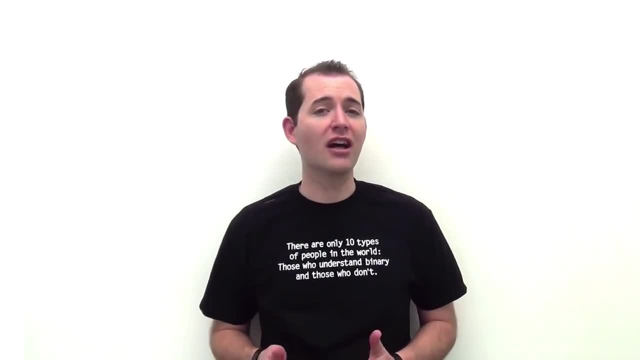 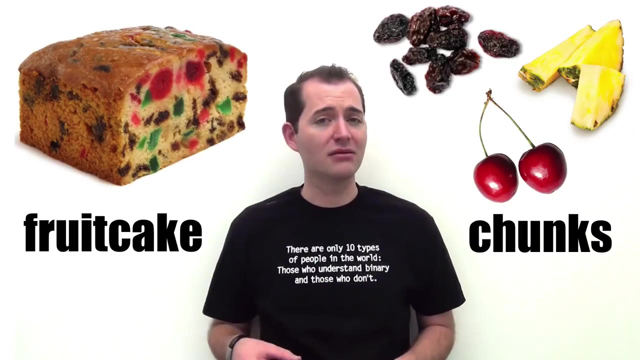 B is younger. This is because rock A had to be around first so that it could be included inside of rock B. An analogy that's similar to the law of inclusions is that of a fruitcake. A fruitcake includes a lot of chunks or other items, and those items or chunks had to be made and bought. 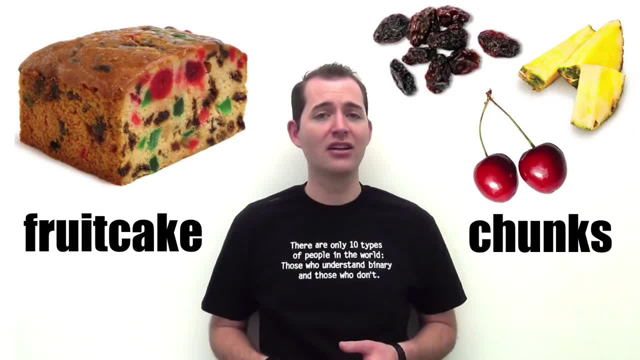 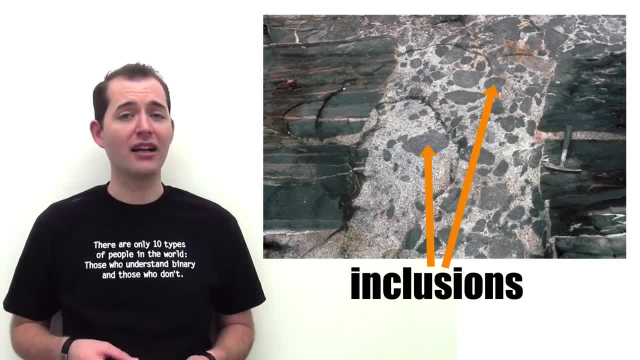 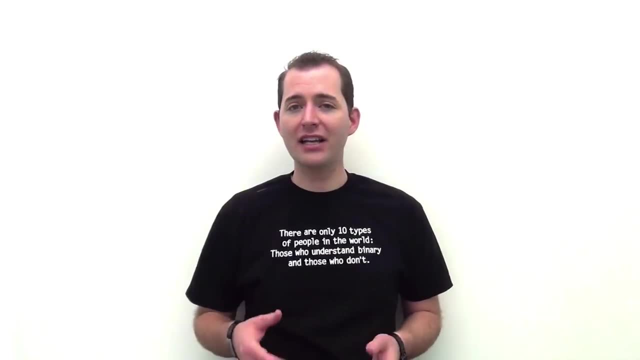 before they could be included in that cake. So what this means is that those chunks are older than the surrounding cake. The same is also true for rocks: Any rock that's included inside of another rock must be the older of the two. Again, we can use these relative rock dating laws to determine the relative or comparative 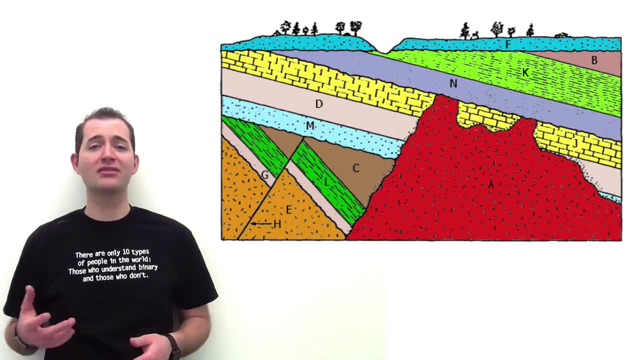 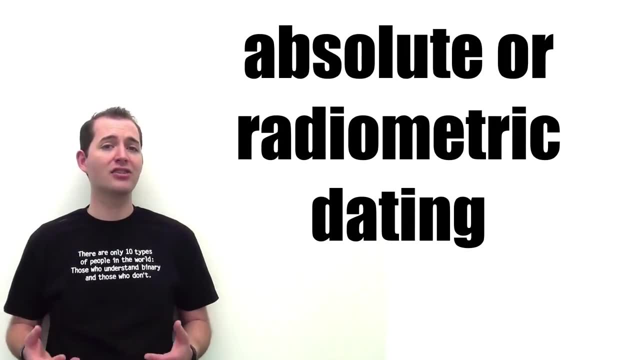 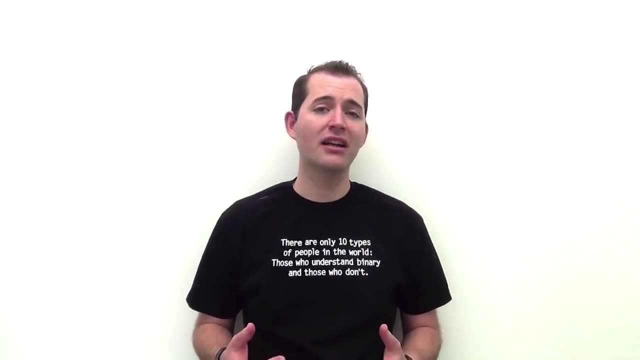 age of rocks to each other. Again, this only means we can tell which is older and which is younger. We must use something else known as absolute or radiometric rock dating to determine specific ages for specific rocks, But these relative rock dating laws are very helpful in helping us determine the sequence. 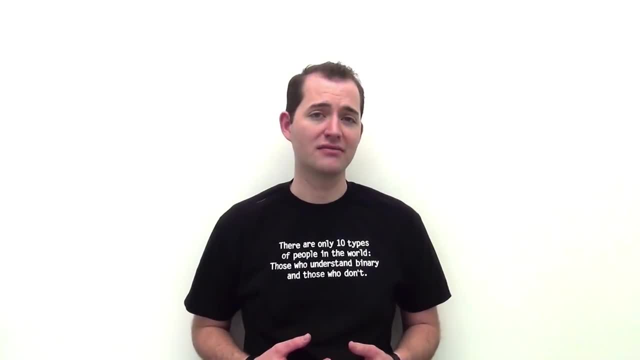 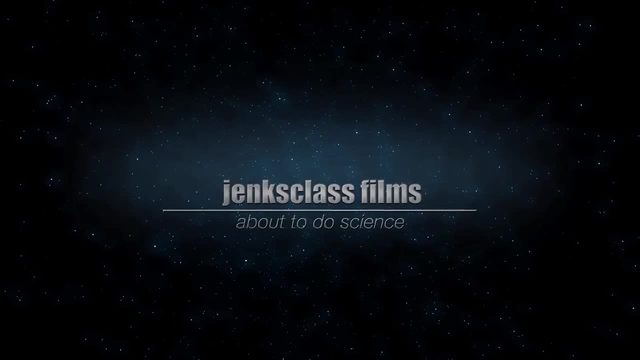 of events that led to rock formation. Thank you for watching.